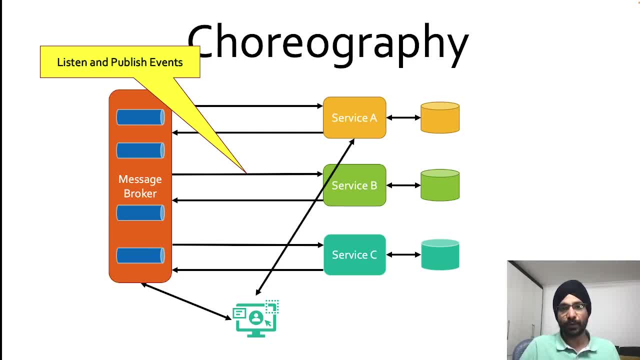 event, or they can directly, you know, initiate workflow in one of these services. let's take one quick example over here. so we have, let's say like no, three services called order service, payment service and shipping service. so how do you really implement this design pattern? so what happen? what? 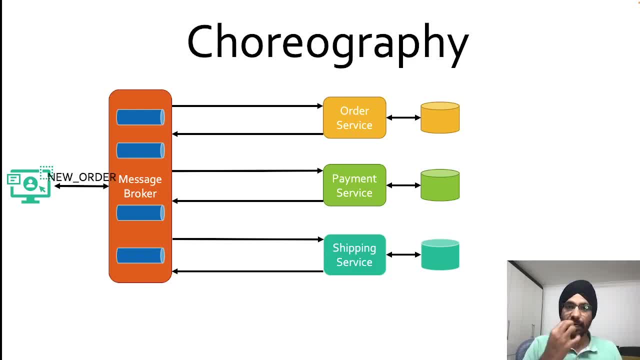 will happen here is: our client will publish a first event saying new order. okay, as i said previously, client can simply publish this event on message broker, on on some specified queue or or topic, or they can directly send to, maybe, order service. but in this example, let's say client is writing: 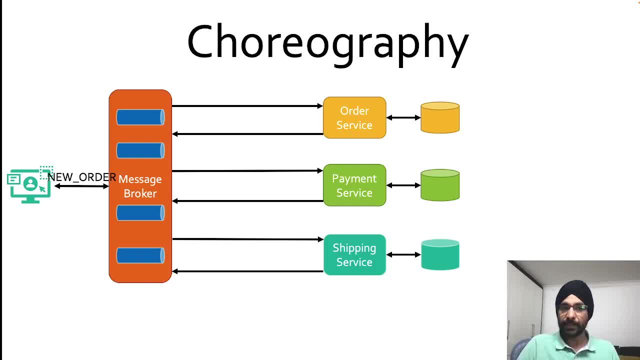 directly to message broker. so, as new order command has been received, an event has been received, let's say order service has subscribed to that particular event. so now order service has consumed this particular event. once order service has completed its workflow, it will reply back with another event called order created. okay, now order created has been published to. 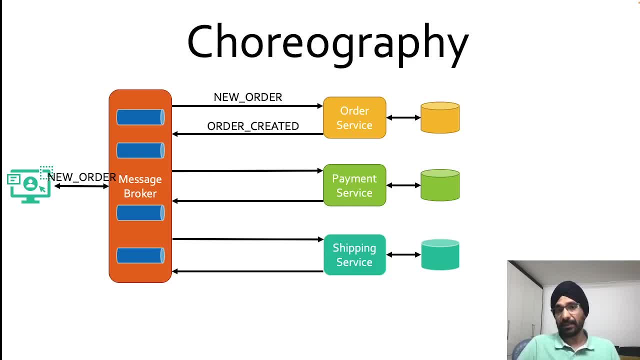 another topic. there can be another service in this particular example. let's say payment service is interested to consume this particular event to drive its, its workflow. so payment service has now consumed order created event. once payment service finishes its workflow it has to publish its own event. let's say: payment received. now another service. 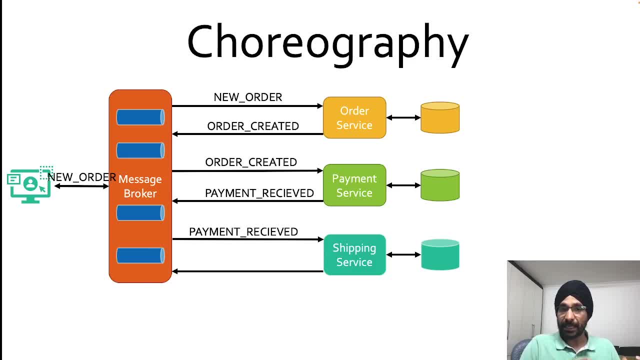 such as shipping service, over here will be kind of subscribing to a topic or queue where the payment received events are published. so now, let's say, shipping service has kind of, you know, subscribe to the payment received, plus also maybe to order created, so it's ready to ship an order. okay, so once shipping service 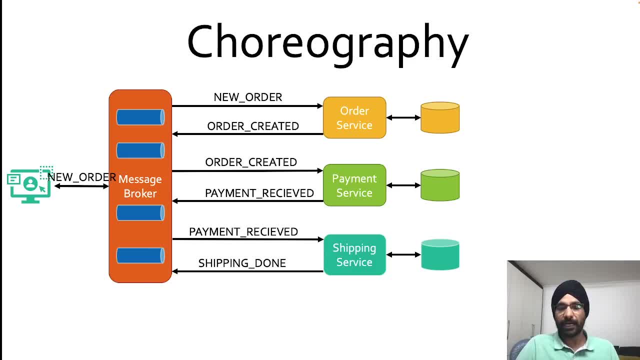 has, you know, successfully shipped an order. what it will simply do? it will create a new event called shipping done, and this shipping done can be sent to client, or maybe it can be consumed by other services to to maybe finally mark their their workflow done. now, let's say hypothetically, there is a little service. 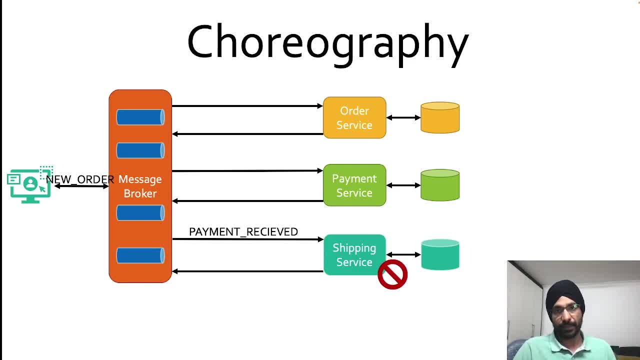 there is a little problem with a shipping service. okay, so shipping service, when it consumed payment received, it cannot fulfill the order. maybe the stock is, is is not there or maybe, like no, they have a some sort of problem with the lorry which is probably going to carry some. 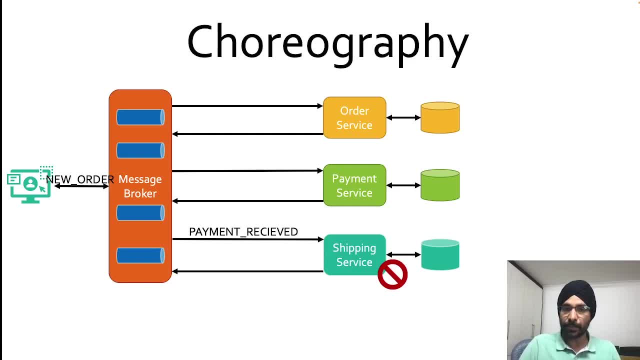 sort of product. so what will shipping service do at this point? shipping service will be initiating an event called shipping failed. it will simply say: that's fine, I receive payment received. okay, I try to ship, but I can't cancel an order now, so I'm going to say shipping failed. so now let's say: 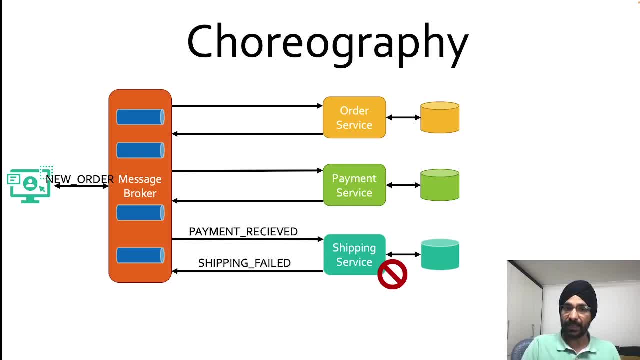 shipping fail and the order service will be initiating a negative or an event which is simply saying shipping field. other services can now subscribe or can listen to topics where this type of events are published. so who will be most interested to listen to these type of failures? of course, payment service. 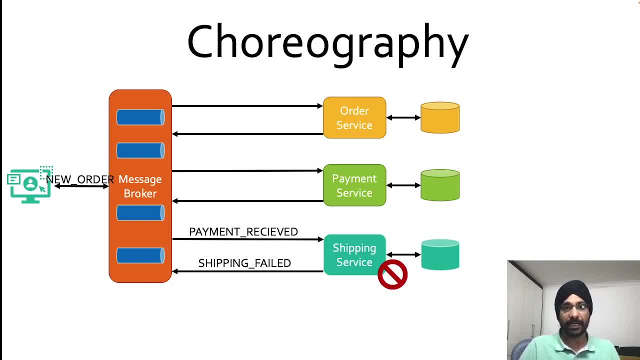 because we have to give a refund to our, our client. okay, plus order service will be. So let's take an example. okay, so shipping failed event came. payment service has rightly subscribed to a topic where shipping failed event was published. So payment service will, you know, kind of will do its workflow and then it will try. 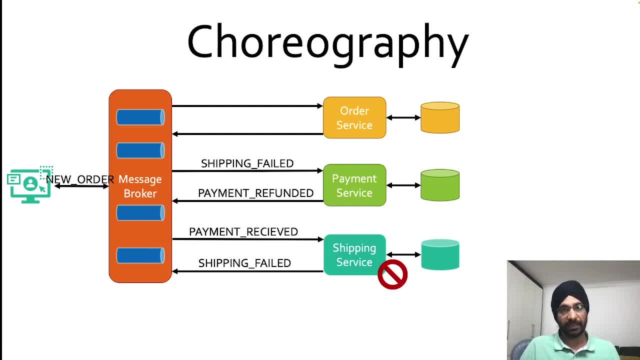 to do the refund and after that it will say: payment refunded. Now, who will be interested to listen to payment refunded? probably order service. So let's say, payments order service is now listening to a topic where payment refund event was published. So after that, order service will, you know, complete its workflow and finally it will 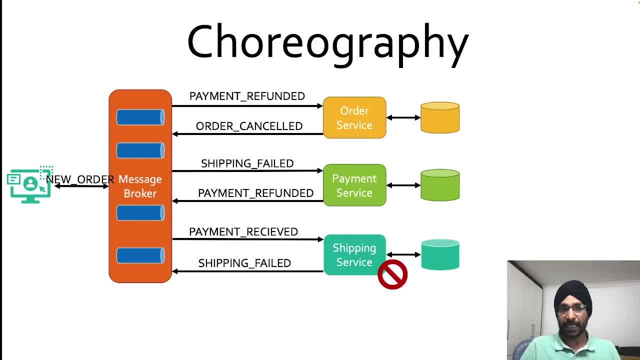 say order has been cancelled. Once order has been cancelled, you know, we can kind of reply back to our client saying your order is not successful. We have, you know, cancelled the order and we have done all the refunds etc. So this is how a choreography design pattern works. 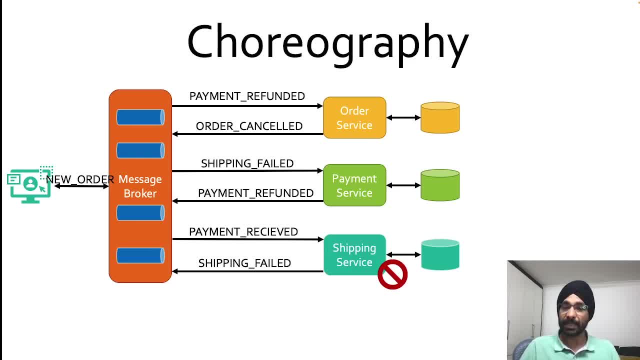 I hope you liked the video. Please give me thumbs up, leave a comment and do not forget to subscribe to my channel. Okay, I will be coming up with new videos soon. Thank you for your time. Bye, bye.